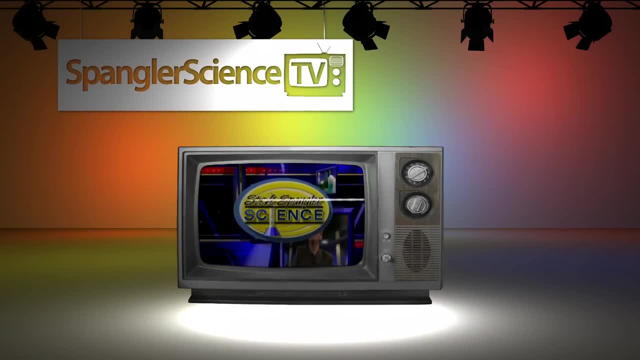 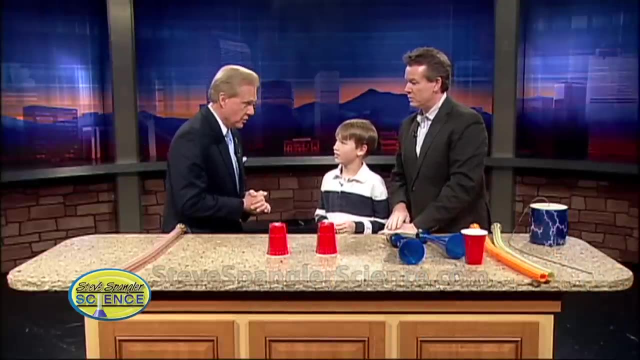 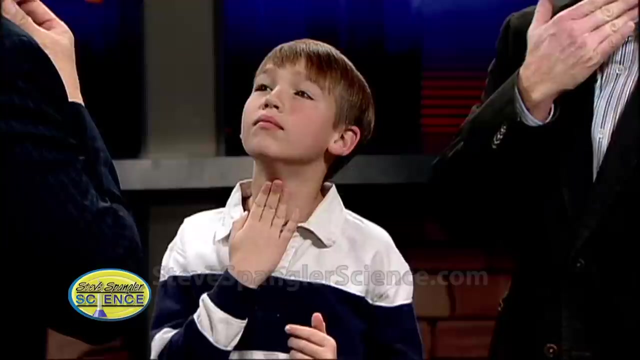 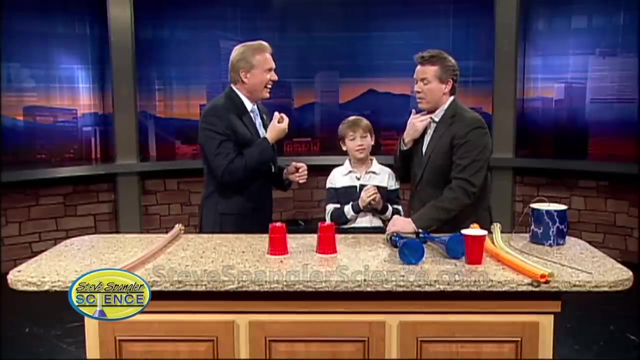 What makes? how do you make sound Vibrations Correct? Nice job, That's really really good. It's on your throat, right. You were showing me before What is that? The Adam sound My larynx? Yep, I feel my lunch. Dad, that's your problem, That is my problem. Show him this. Would you show him? because you were playing with the cups, so show him this. So this is how I make sound. 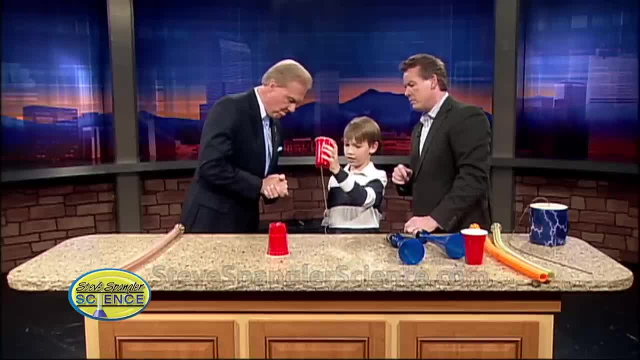 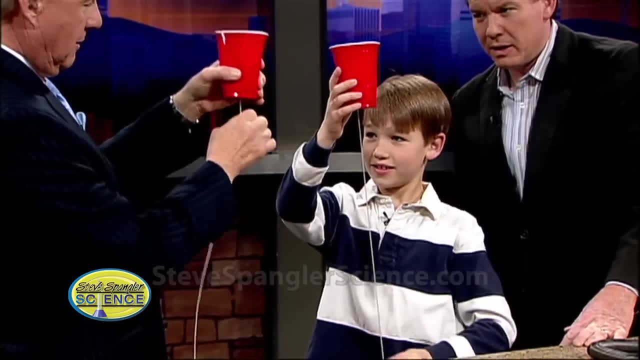 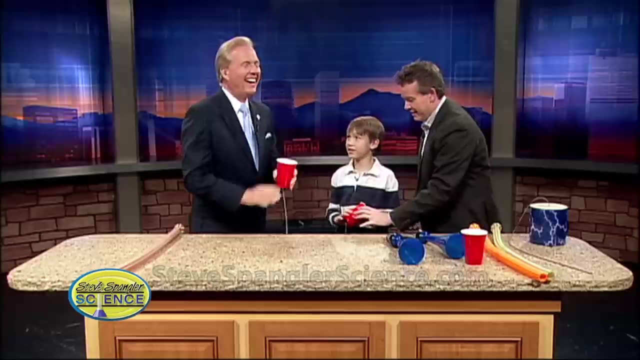 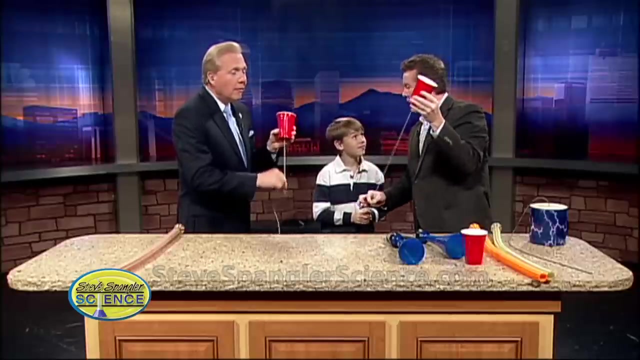 So this is how you make a homemade thing. It just takes a red cup and a string. Good, And he has one here. that's yours as well. Oh, excellent. So now here's what you do. What do you do? Pinch it and pull down. Oh nice. What does mommy call this? The most annoying sign experiment Of all time? right Of all time. The secret is stick and slide. So it's a chicken cup. It's a chicken cup like a stick and slide, So that's kind of a fun way to be able to do it. We should have our own show, you and I. 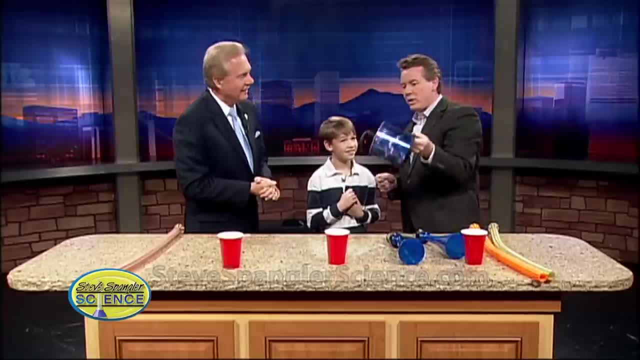 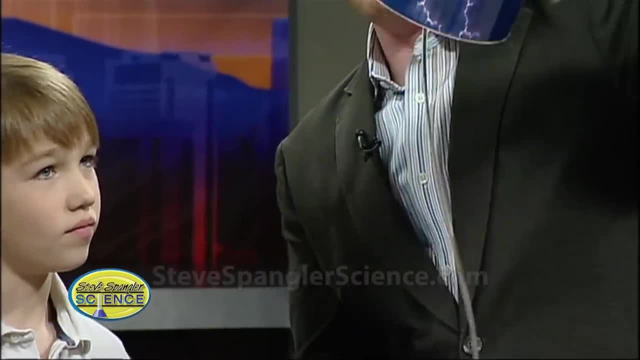 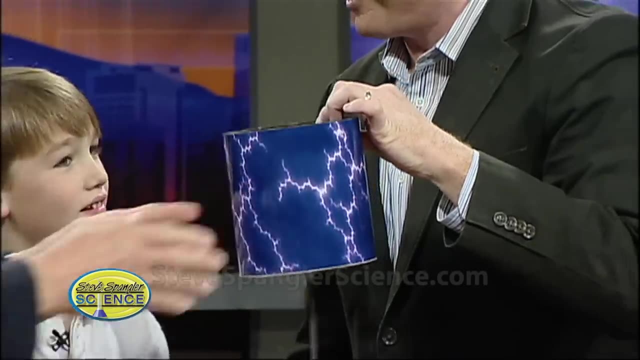 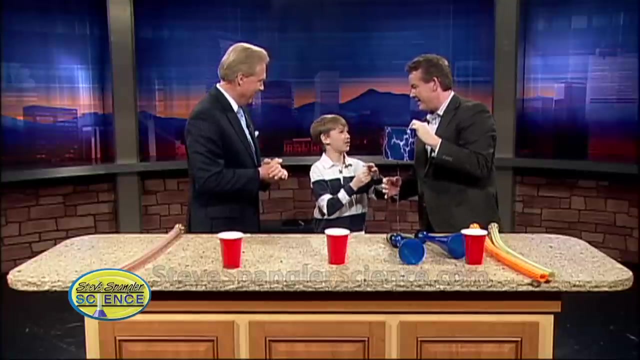 That's good, But this is what you can find at the toy store. So instead of using a cup, they're using kind of a little barrel that you see here, and there's a spring instead of a string. Fair enough. So when we pull this here, watch what happens when we pull this. Oh, much better. Kathy Saban would love this one, don't you think She would love that? Yeah, Is this a great one? So what do we do to trick people? We always put it on the phone, say we're outside and it's raining, but it's really just a sunny day. It's just our vibration. It creates our sound. 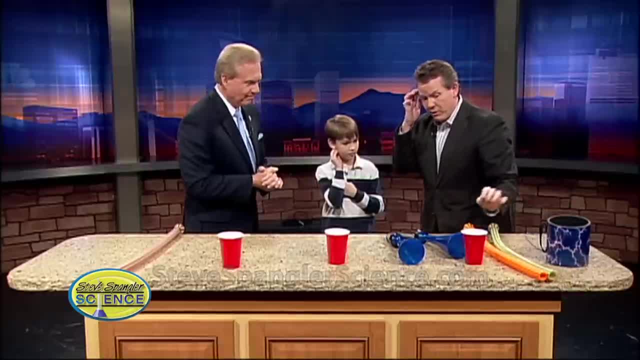 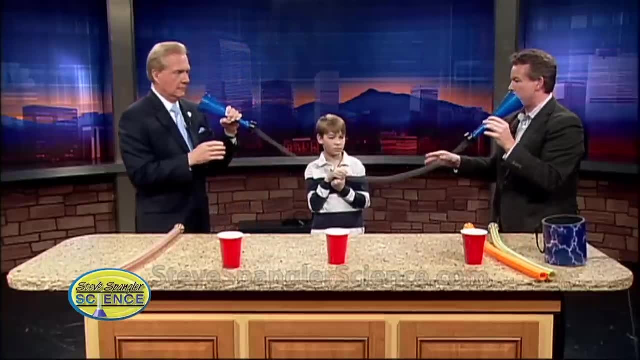 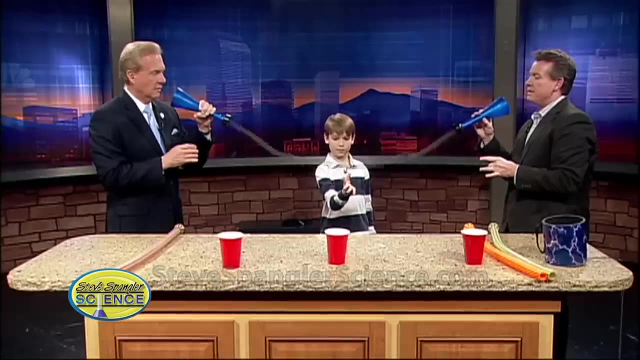 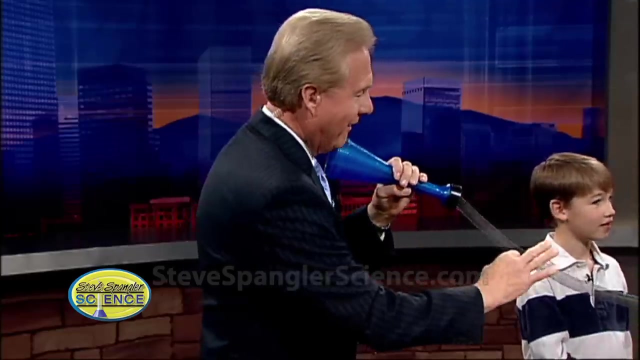 Is that kind of fun? No, this kind of translates into this was very fun because they used it for special effects. Look, there's a horn on each side. So, Mark, you're going to be on the side, You and I are going to stretch out just a little tiny bit right there. That's perfect. And now listen to this. See the vibration here, the spring. Watch what happens when little Mark snaps it. Listen, Isn't that fun. Oh, that is really cool. This is what they use. Oh, there it is. This is what they used for the first little. I had things in Star Wars. They said the special effect was there. Isn't that kind of fun? Vibration in the spring. 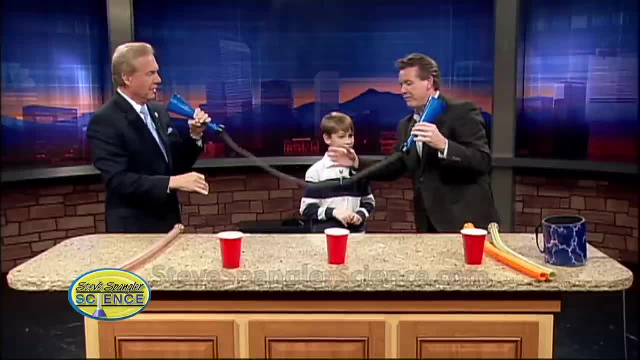 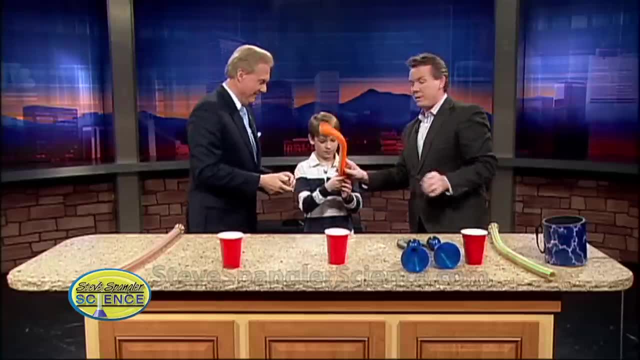 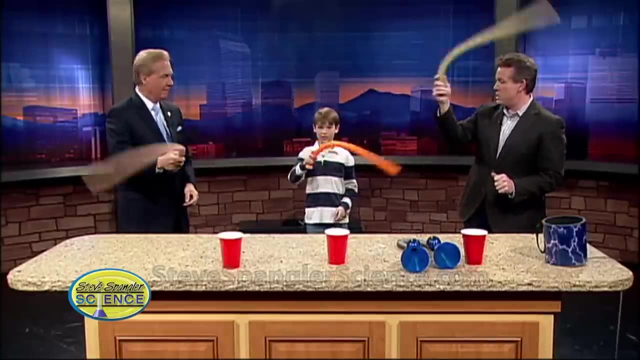 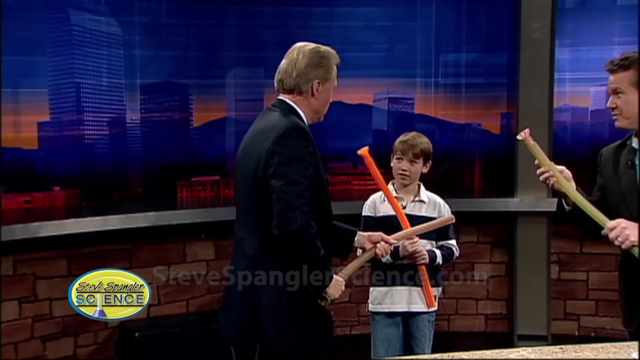 Sound Lightsaber: Yeah, Shooting, Not very technologically advanced, but it works because it's the vibration going on the spring. That is very cool, All right. but our favorite one, Mark, you've got to show them this and hopefully nobody gets taken out. That's yours, Mark, All right. So what do we do here? Spin it around, Listen to this, Listen, Okay. try to stump him and ask him how he thinks it works. How does this work? Well, it must have something to do with the speed of the air through the tube. He's got a PhD in physics. I love that. 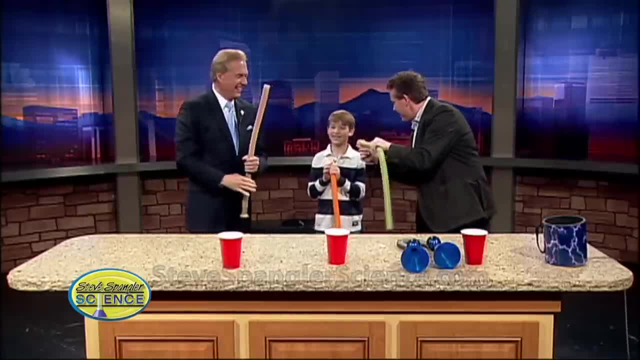 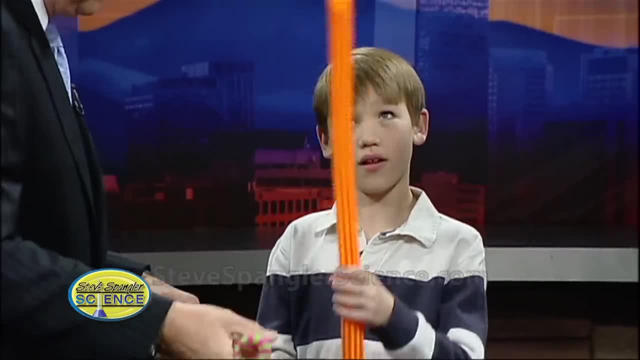 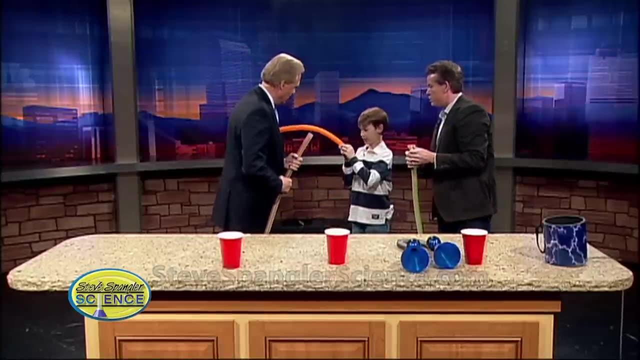 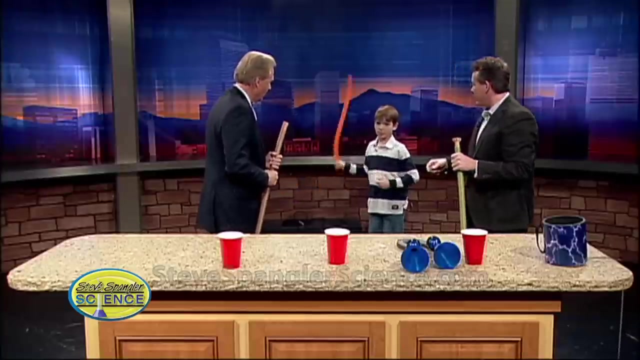 What's inside? Years of spangler science. ladies and gentlemen, What's inside, Mark? Tell them what's inside. What are you doing? So, really, the molecules will go in one end and when you spin it, all these ridges here make the molecules tumble and then they come out the other side. But here's how we prove it. You are a young genius Here. watch this. Do the cork and then we'll wrap this whole thing up Ready. So this cork goes in. so now the air can't get in there. Now listen to this. See, it doesn't work Nothing. Take the cork out and see if you can make it work. Ready, Now go for it. Oh, Nice way. All right, you and I are going to do this. Can you buy these two? I think, Yeah, it's all the toy store. You know it's the toy store. 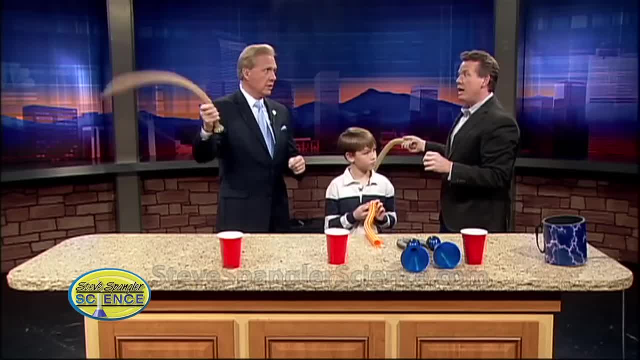 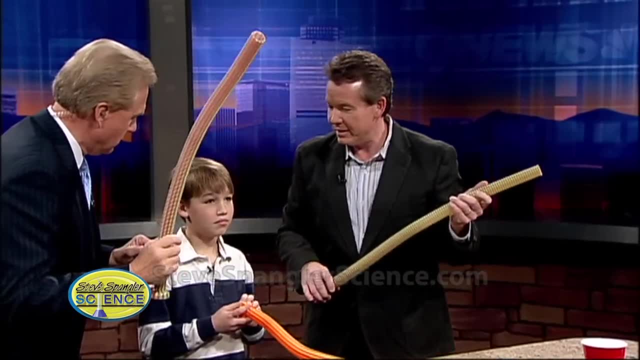 The toy store and online and all that kind of stuff. As you know, the young, the grandkids, would love that. That's exactly right. They'll always take Grandpa out, though, so you're going to come to work with a little smack on your head. What does Mom say about this noise? Does this bother her less? I don't know. Yeah, well, That's how it works. We'll have to test that one out. You tell them about the website. We'll serenade you for it.